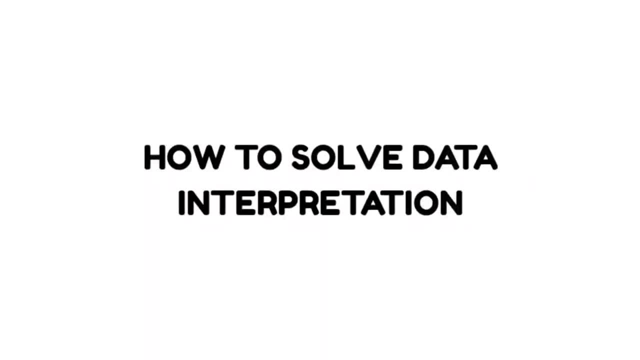 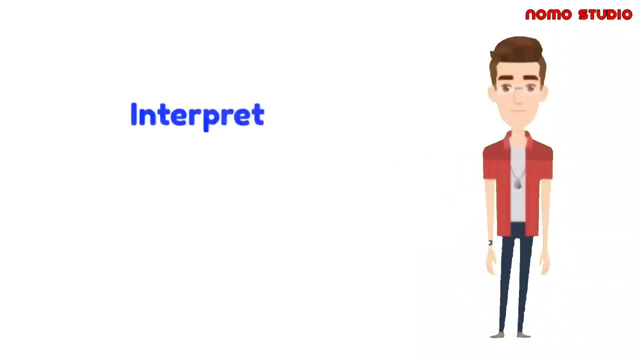 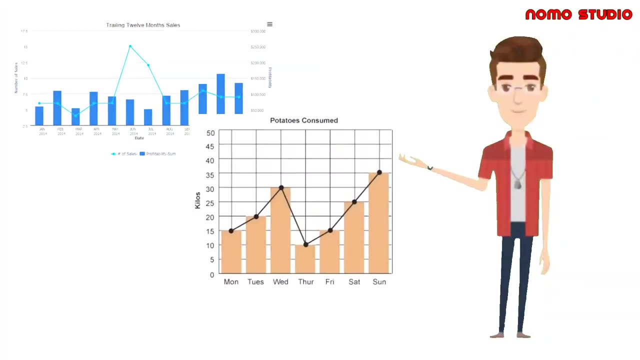 Many jobs require employees to be able to interpret, analyze and make strategic decisions based on data, which is commonly presented in charts, graphs and tables. Data interpretation questions, which often feature in numerical reasoning tests, assess someone's ability to interpret mathematical data. 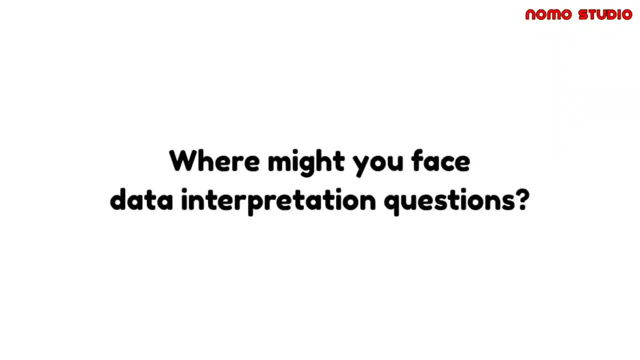 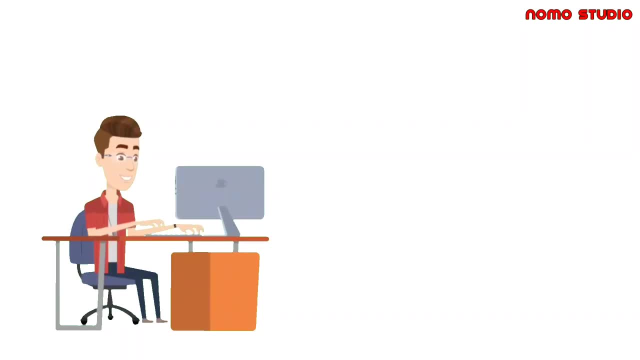 You may also expect to face a data interpretation test if the role you apply for includes any data analysis or strategic decision-making or data handling. This could include marketing, clerical and administrative roles, as well as managerial positions where you will have decision-making responsibilities. 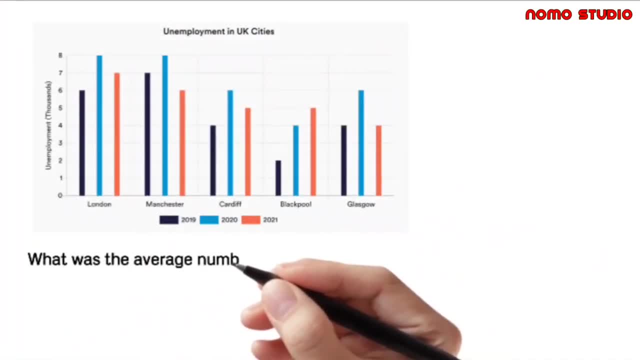 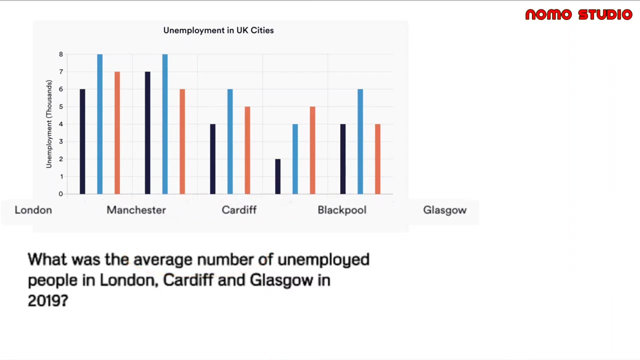 What was the average number of unemployed people in London, Cardiff and Glasgow in 2019?? Observe the given data. the question focuses on average. These are the cities in United Kingdom with given number of unemployment. Color: black for the year 2019, blue for 2020, and orange for 2021. 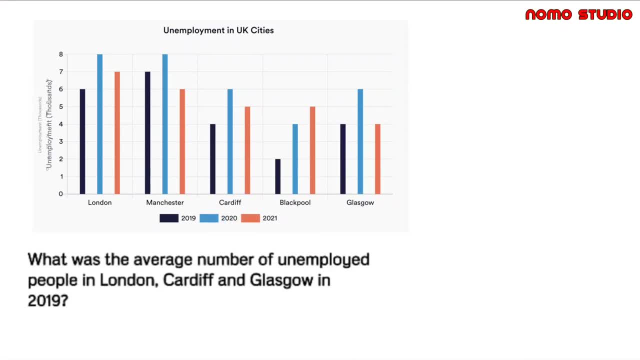 What was the average number of unemployed people in London, Cardiff and Glasgow in 2019?? Numer of unemployment is given in thousands, So meaning one stands for one thousand, two for two thousand and so on. Any word I leave unanswered. 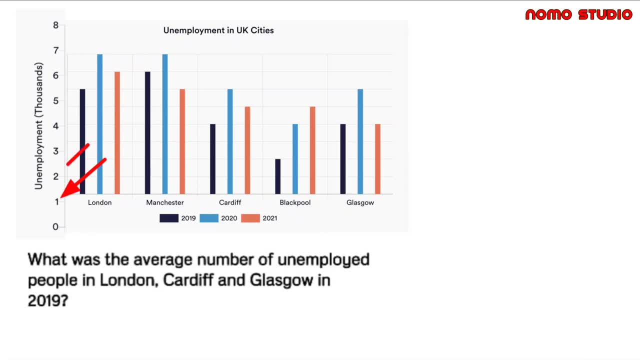 You should think about which one is right. You can find them in the workbook on the website. If you can not distinguish, you can die. The target price is which Write in the comments. The number of unemployed is given in thousandths, so meaning one stands for one thousand, two for two thousand, and so on. 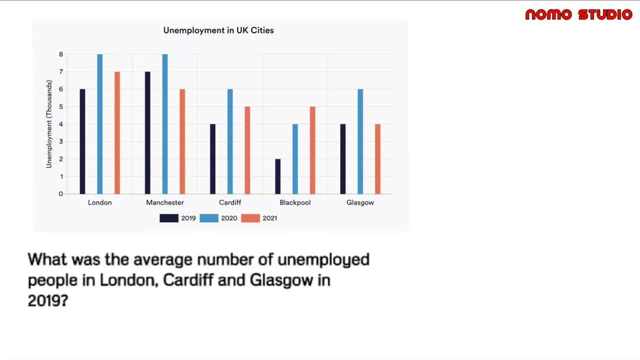 Now get to the question. we only have to focus on 2019.. Noted down the figures for these cities in 2019.. By consulting the key at the bottom of this graph. If you look up the graph, you will see. you need only the black figures. 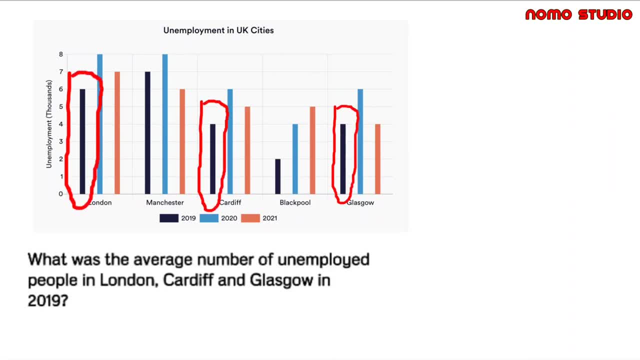 The photos are match black columns by city. we only need the column for London, Cardiff and Glasgow. so we have 6,000 for London, 4,000 for Cardiff and 4,000 for Glasgow. let's add them up: 6,000 plus 4,000 plus 4,000, which is equal to 14,000. 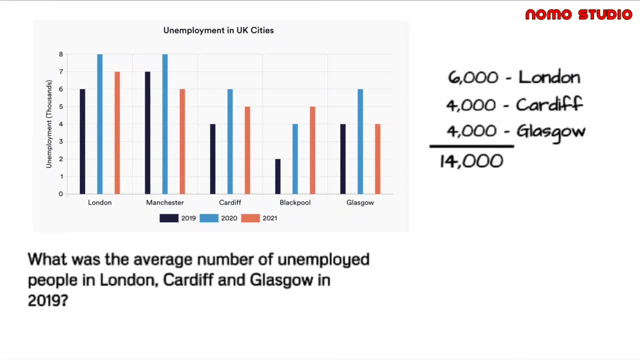 now, since we are looking for the average number of unemployment of the three cities, let's divide 14,000 by 3, so the quotient is 4,667. therefore, the average number of unemployed people in London, Cardiff and Glasgow in the year 2019 is 4,667. 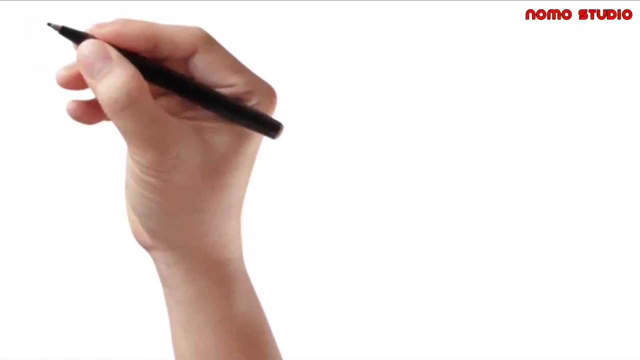 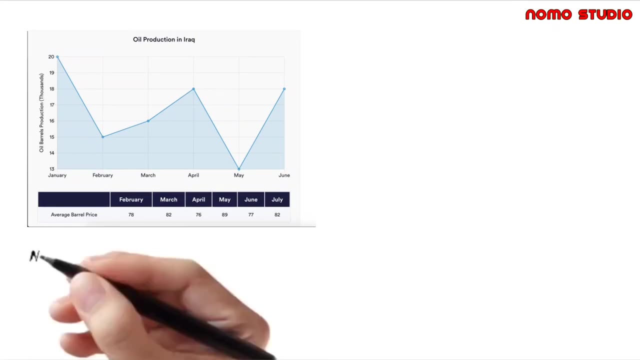 you. example number two. consider this graph. the question is: what was the percentage change in the value of oil produced from April to May? this question looks of oil production in Iraq, which is set out using a graph measuring months from January to June. it also shows the number of oil barrels. 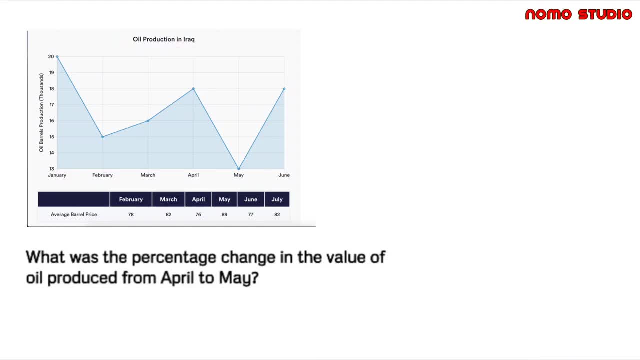 produced and the average barrel spent on the oil production in the country. barrel price: Remember that you are only asked to calculate the percentage change in the value of the oil produced from April to May. These are the average barrel price from February to July and these are the oil barrels production in thousands. 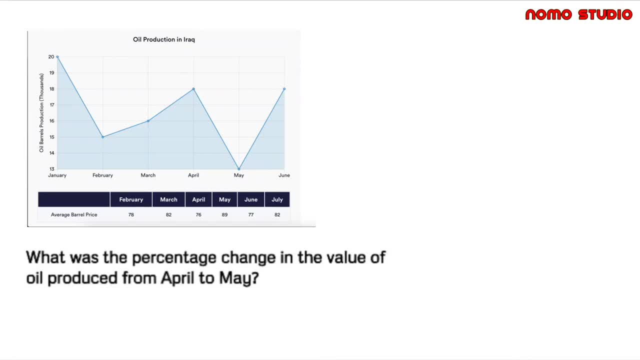 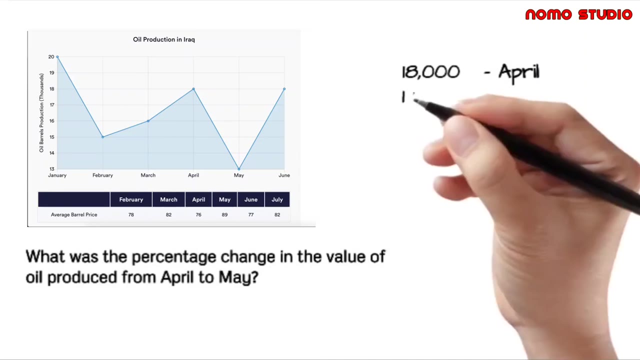 Note that you will need to look at only two months of data, which is April and May. Let's identify the production amount for April, that is 18,000 barrels. Then the production amount for May is 13,000 barrels. Let's calculate the value of oil produced for April using the chart at the bottom of the table. 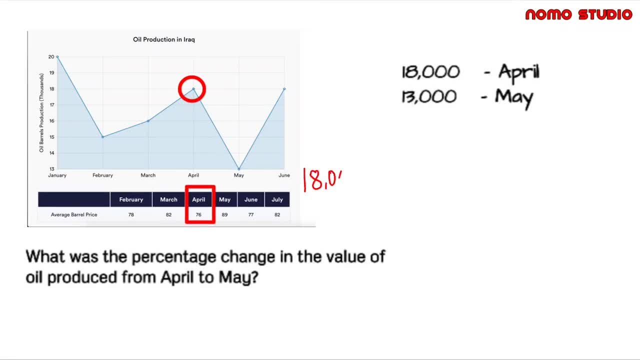 18,000 barrels multiplied by $76 average barrel price, and that is equal to $1,368,000.. Let's also calculate for the month of April: 13,000 barrels multiplied by $89 average barrel price, and that is equal to $1,157,000. 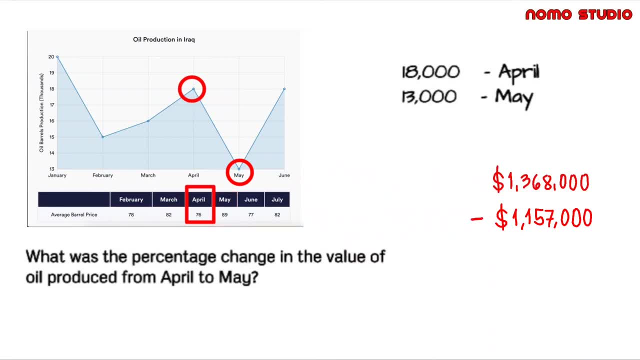 Next is work out the difference in value of $1,368,000.. For the month of May, we will divide it by $2,171, and also the $1,157,000,, since we are looking for the percentage change.